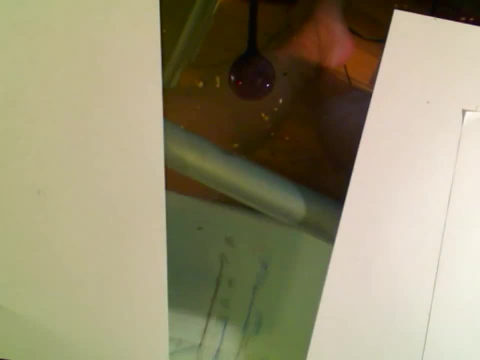 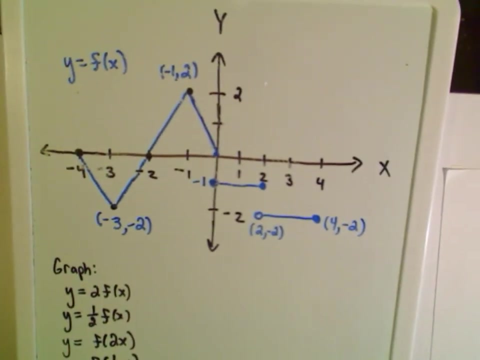 Okay, so I'm going to do one real generically here. I've got a real generic one here that I'm going to do, And so this blue function is my function f of x, and these are all supposed to be straight lines. 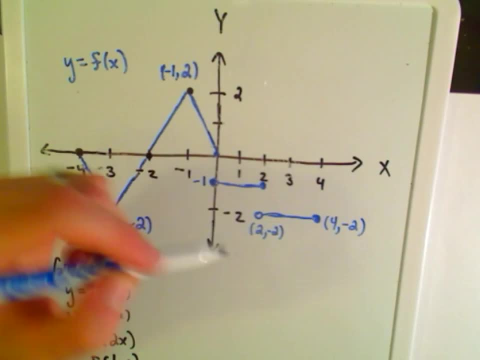 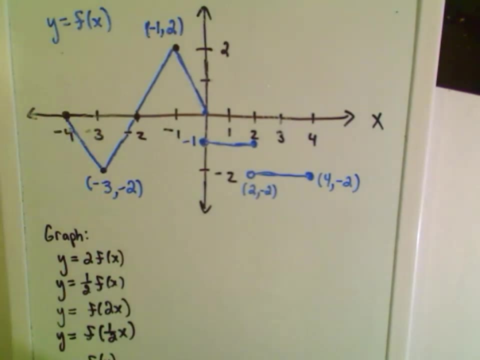 Okay, and eventually I'm going to do some other videos where I put all of this stuff together and some more complicated ones, But for now just kind of the bare bones. Okay, so it's kind of this little sawtooth function on the left-hand side. 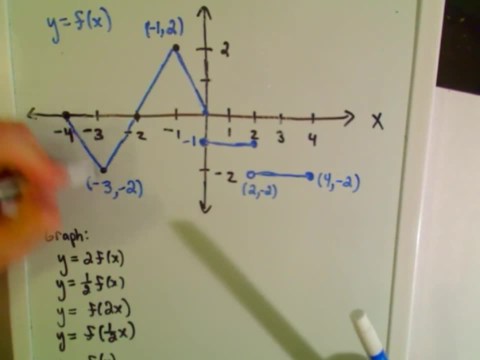 It's got an x-intercept at negative four. When it's at negative three, it's down here at negative two. When it's at negative two, it goes through zero. When it's at negative one, it's up here at positive two. 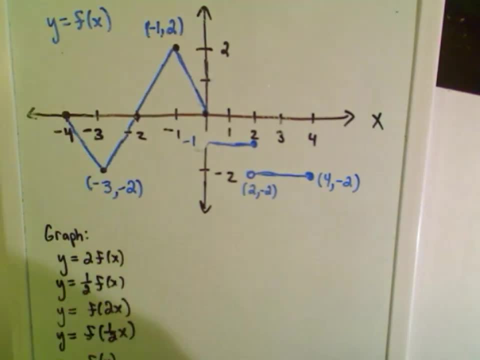 When it's at zero, it's at zero. It should be an open circle here. At negative one, and then it's just supposed to be a flat line extending over to two. And then it jumps down. It starts at two negative two, and again is a flat line from four to two. 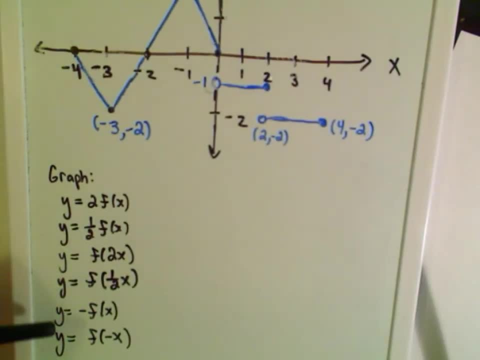 So what I'm going to do is I'm going to graph all six of these functions that I have down here on the bottom left. So two times the function, a half, the two inside, the half inside and a negative out front, and then f of negative x. 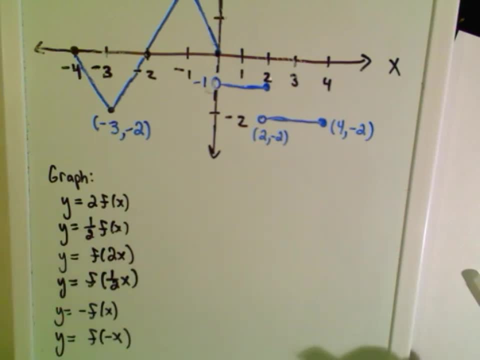 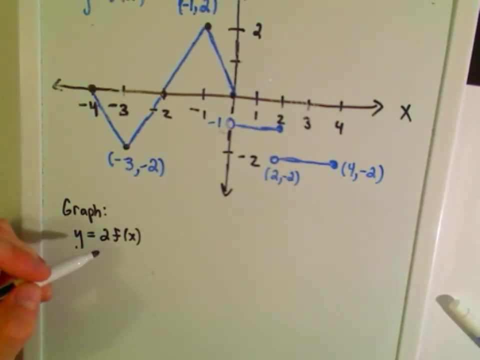 So let me see if I can. Let me do them all here. All right, so let's do the first one first. Okay, so I'm going to try to graph what two times this function would look like based on the original function. 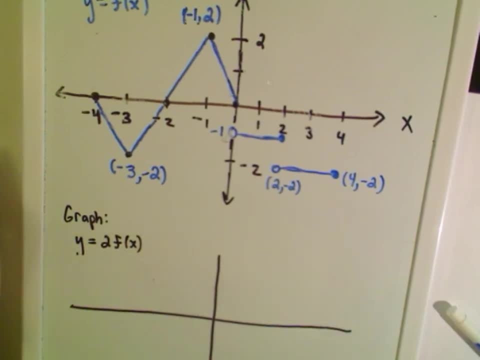 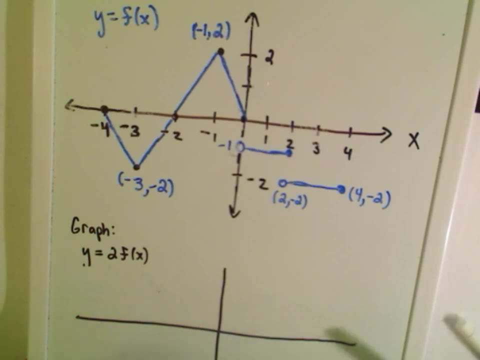 Again, there's no way I'm going to be able to get through all of these in one video. But basically what happens is if you take two times the function, what you're really doing is you're multiplying. Think about f of x as being y. 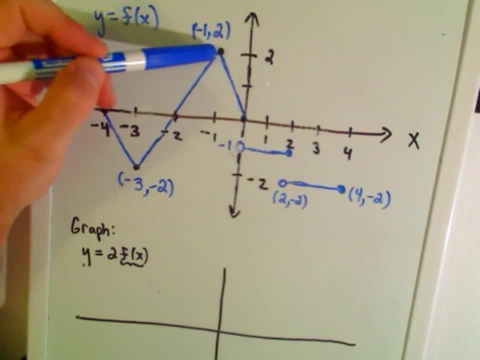 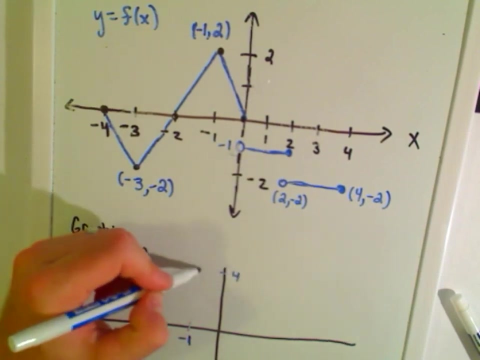 You're multiplying all the original y coordinates. You're multiplying all the original y coordinates by two. So instead of you know at negative one, instead of being at the y value of two, you're now multiplying it by two, so that you'll be up here at a height of four. 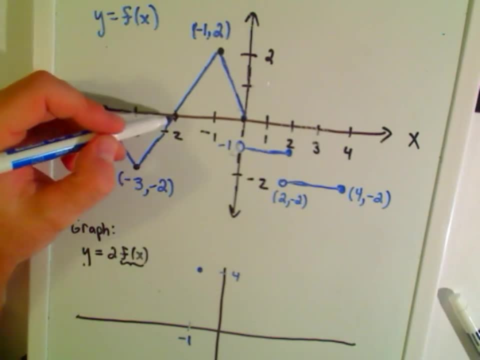 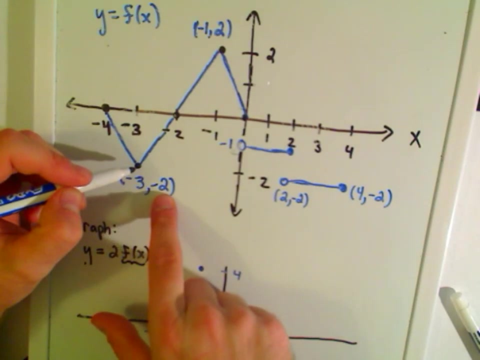 Okay, if you think about the x coordinate of negative two, its original y coordinate is zero. If you multiply that by two, well, you're still at zero, At negative three. originally your y coordinate was negative two, But now, if you multiply it again by two, you're going to be down here at a y coordinate of negative four. 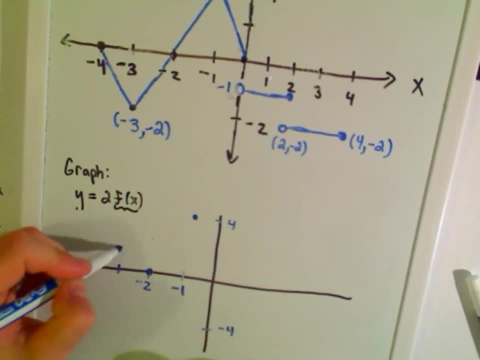 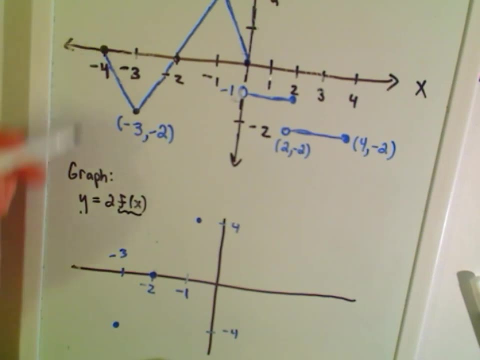 Let me see if I can squeeze it in here. So here's negative three, Again a real rough graph. Sorry, I'm not an artist. And then at negative four, my original y coordinate is zero If I multiply that by two. 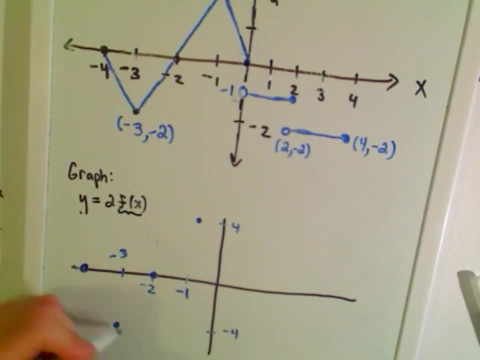 well, I am still at zero, Okay, and then it's still going to have that sawtooth shape associated with it. Okay, again, it doesn't really look like it, but it's supposed to be stretched out. Look where the y coordinate is now. 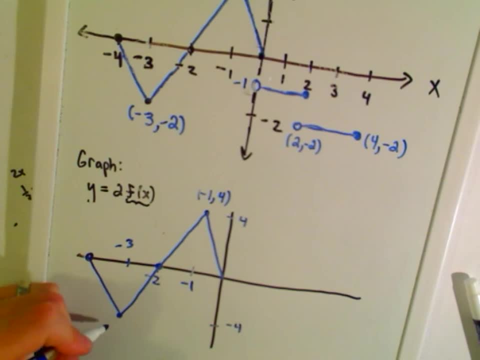 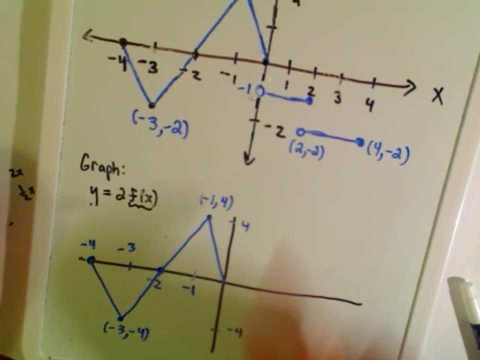 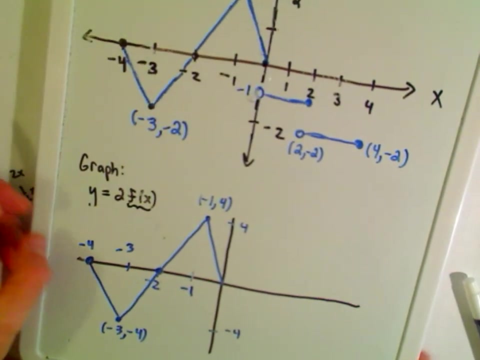 This is negative one comma four, And down here at the bottom left this is negative three comma, negative four. It's still a y intercept of negative four. On the right-hand side it's going to have the same effect. It's going to multiply the original y coordinates all by this value of two. 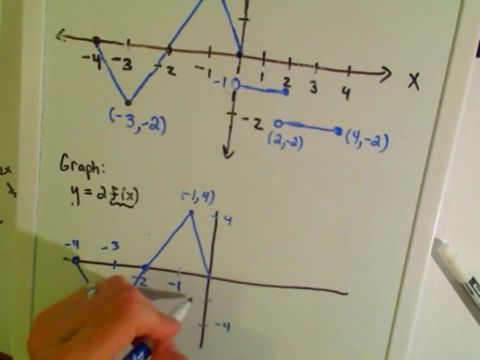 So, instead of being at negative one, it'll now be at negative two. It'll still extend over the same distance And then it'll jump, And again, instead of being at negative two, it'll now be down here at negative four. 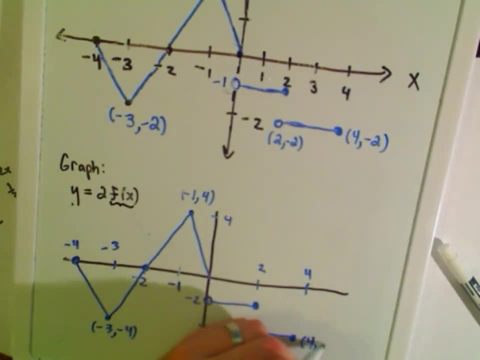 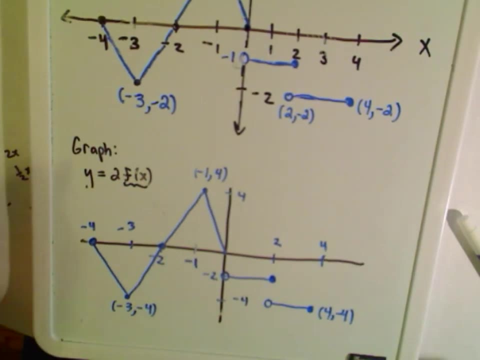 And will extend over a distance of four units as well. Okay, so that's the basic idea here. When you multiply the function by a two, it just stretches everything out by a factor of two. Okay, sorry, let me try to bring it back into focus here for a second. 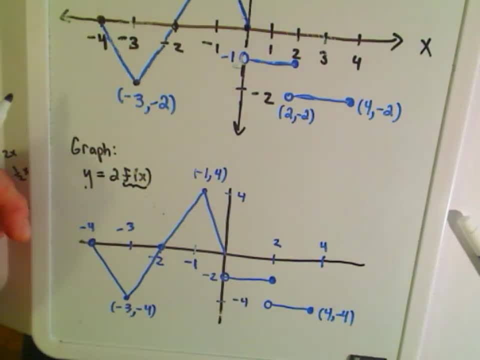 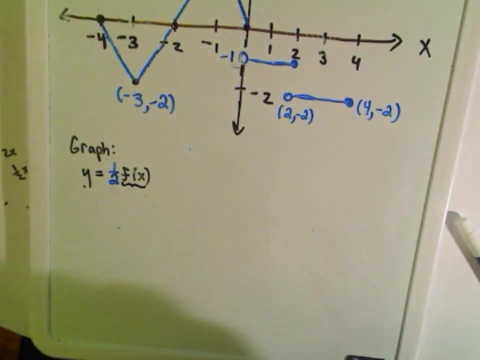 Okay, so hopefully that's a little better. Alright, let me see if I can at least do one more in this video. Instead of multiplying it by two, suppose we multiply it all by one, half out front. Okay, it's going to have the exact same, well, I guess. obviously not the exact same effect. 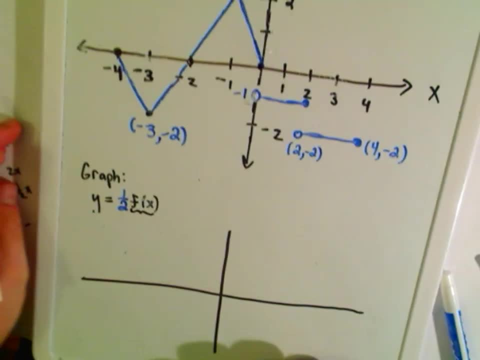 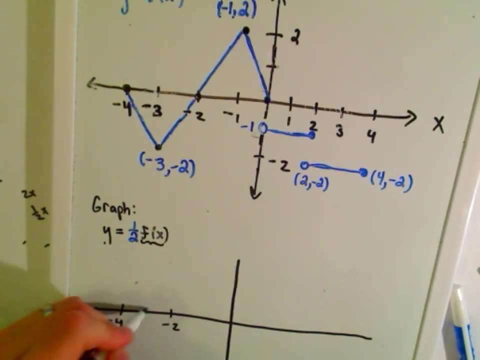 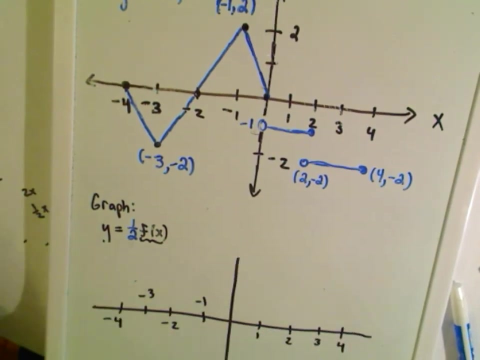 but the idea is the same. It's still going to go out the same distance. It's still going to go out to negative four, Okay, and it's still going to extend out to positive four on the right-hand side, But the difference now being is I'm now multiplying the y-coordinates by one half. 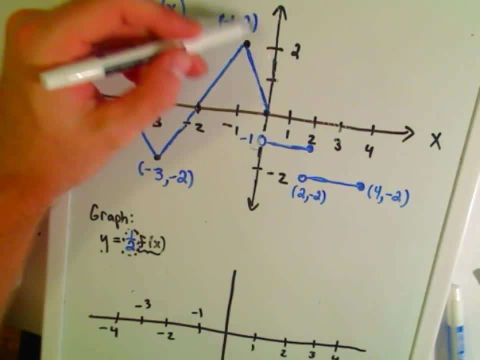 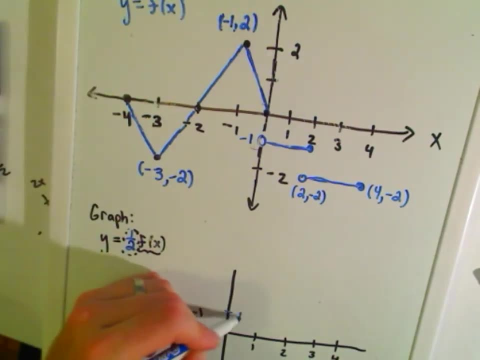 So all of the original y-coordinates are now going to get multiplied by a half. So instead of being at negative one comma two, I'm only going to go up a distance of one now. So I'll be at negative one comma one. 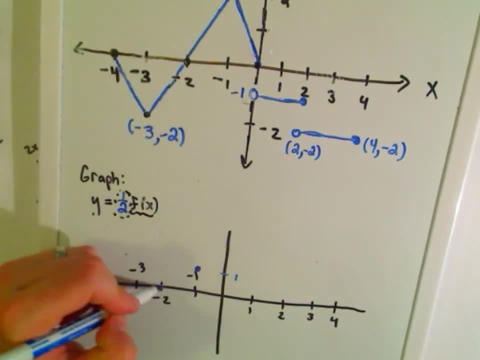 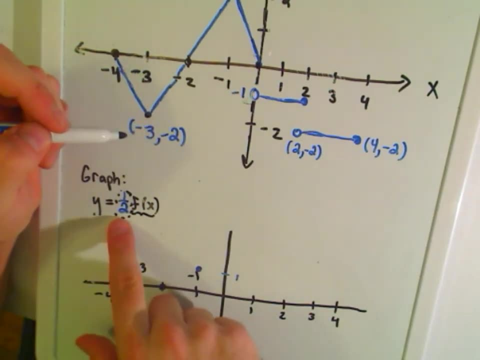 The original y-coordinate associated with negative two was zero. so I'll still be there. The original y-coordinate associated with negative three was negative two. Again, if I multiply that by a half, I'm at negative one. The original y-coordinate associated with negative four is zero. 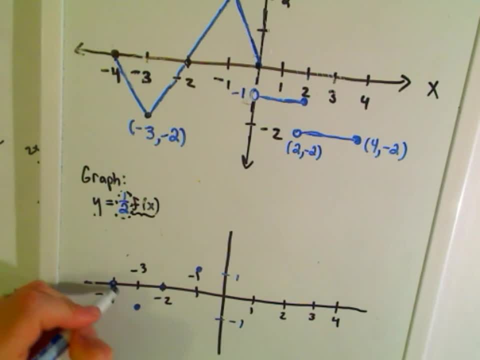 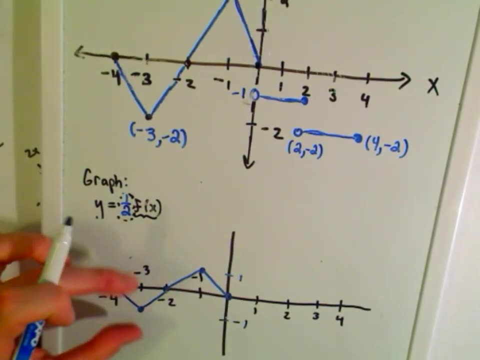 If you multiply that by a half, again you're at zero. So I think this one does look a little bit better maybe than my last one. It does look, I think, a little more squished. So I multiply the function by a number smaller, basically a fraction between zero and one. 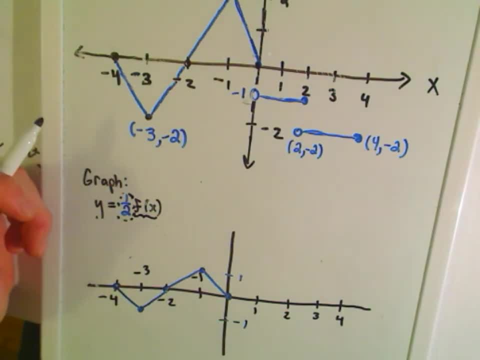 and it's going to squish the graph, It's going to compress it. It's going to compress it vertically. On the right-hand side, the same thing is going to happen. Instead of going down to a height of negative one now, we'll simply be down at a height of negative one half. 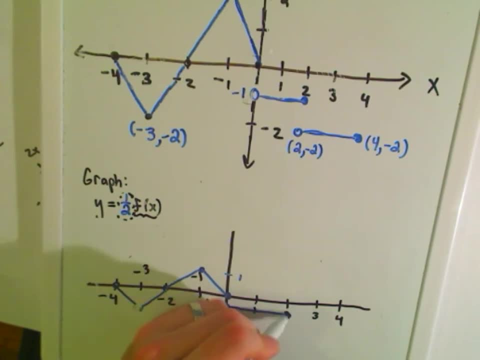 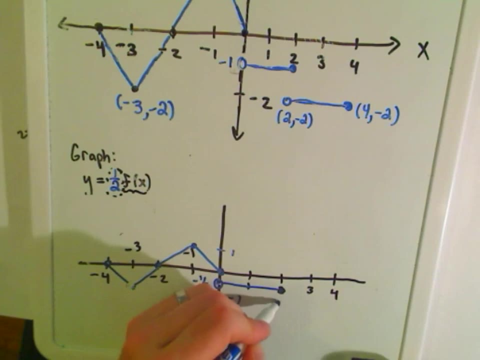 Open circle. It'll still be a flat line over to two. Okay, it's getting a little covered up. And then at two. instead of being at the y-coordinate of negative two, we'll now jump down here to negative one. So this is two comma, negative one. 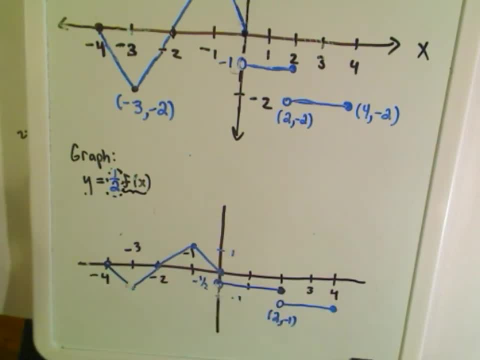 And then that line will extend all the way over. It'll bend all the way over to four. Okay, and that would be the graph of one half times the function. All right, so I'll try to do the other two in one other video. so dig around for that. 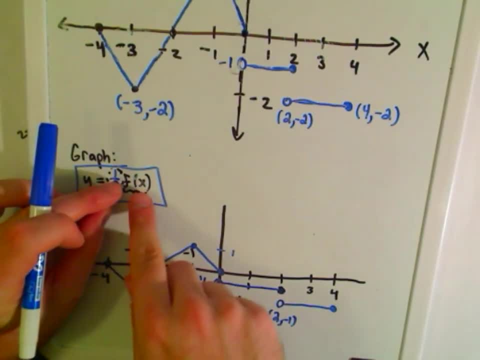 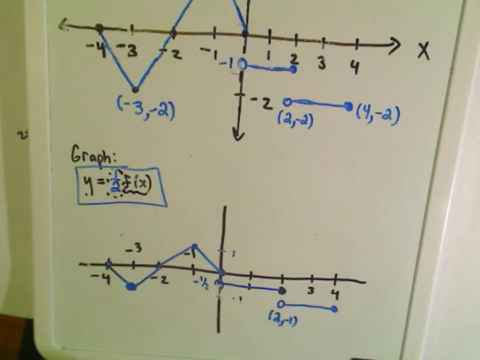 I'll do f of where the two's inside, where the one half is inside, and then we'll do a reflecting of about the x and y-axis as well.